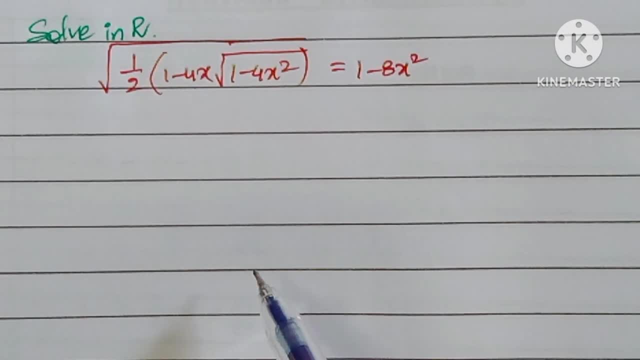 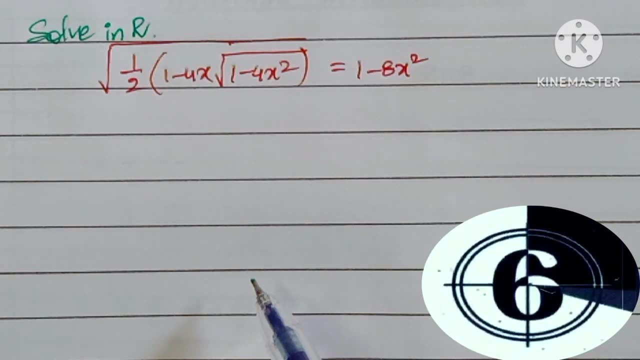 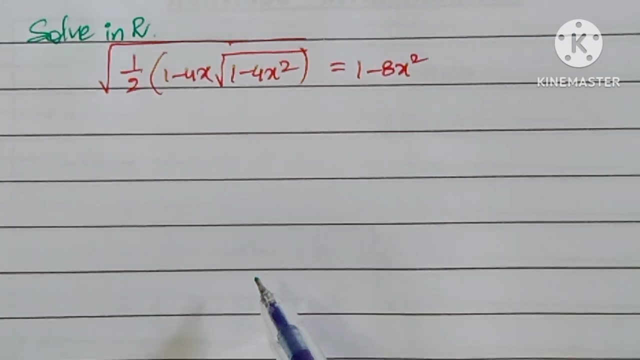 uh, logical and olympiad problem. pause the video for 10 seconds and try it. okay, and also, if you are new to the channel, please subscribe the channel and give it a thumbs up. it will appreciate us to make more videos. more than thousand olympiad and logical problems are. 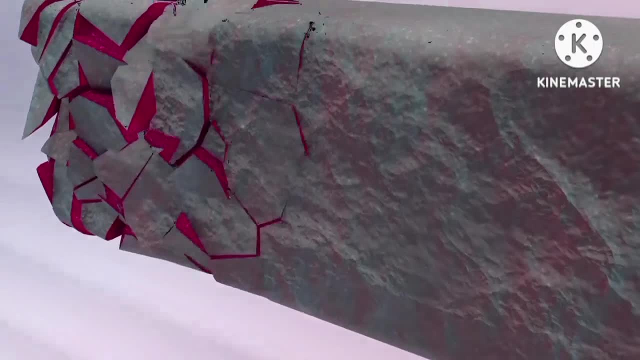 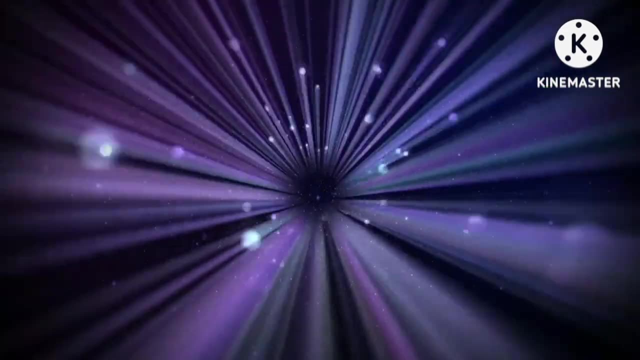 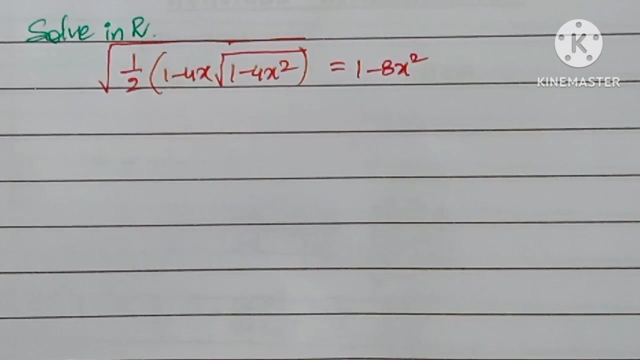 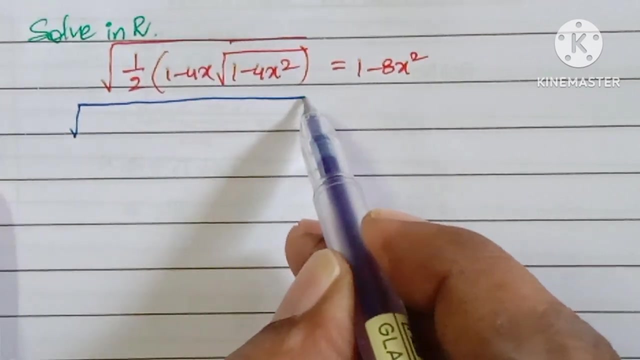 uploaded in this channel. please go through them. thank you. how to solve this? so you can do by squaring on both sides, but uh, it will be somewhat difficult. uh, you are going to another way, how to solve this problem by adjustment, so here i will send this. 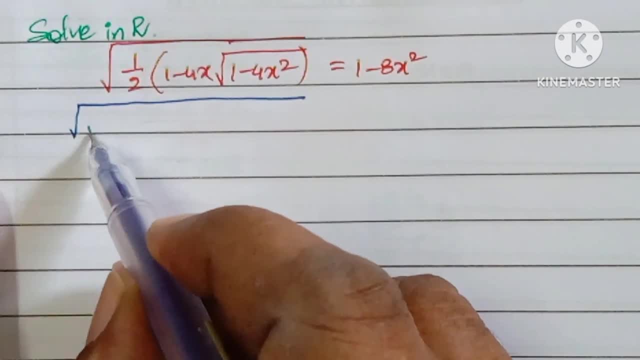 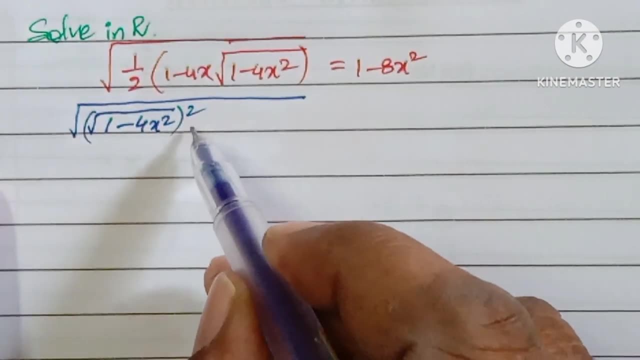 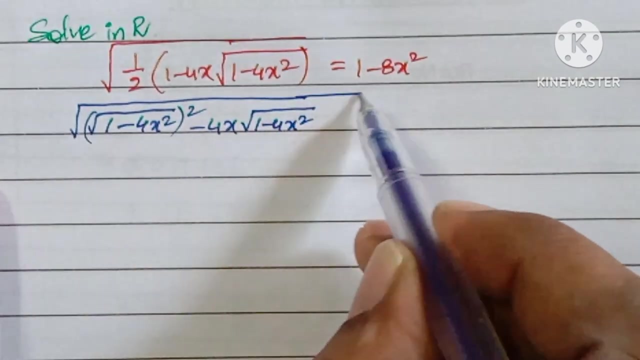 uh, root to that side. so the remaining i am writing as root of 1 minus 4 x square, whole square minus 4 x. root of 1 minus 4 x square. here i have and 4 x square subtracted 4 x square here. 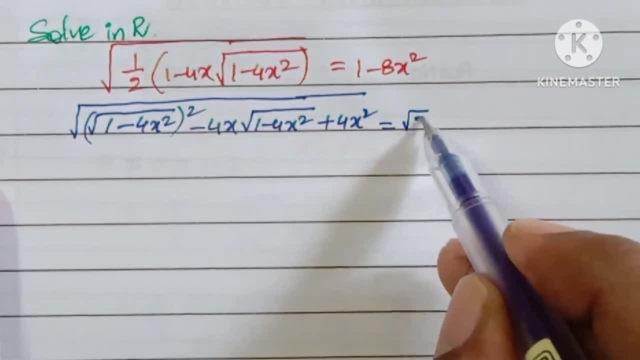 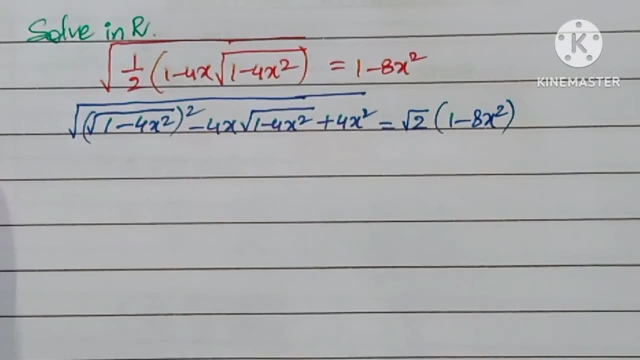 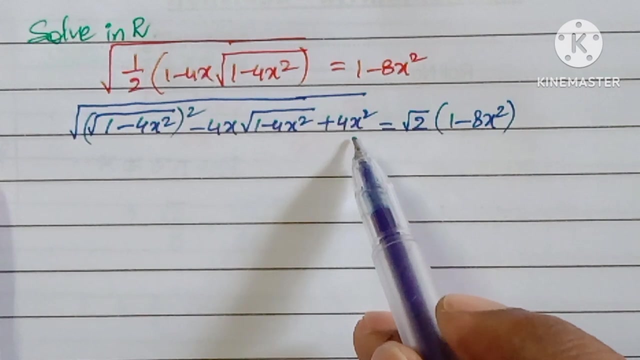 and adding 4 x square, the value won't change root 2 into 1 minus 8 x square. root 2 is taken to that side. now, here it is in the form of a square minus 2, a, b plus b square. a square minus 2, a, b plus b square. this is a value and this is a. 2x is b value. 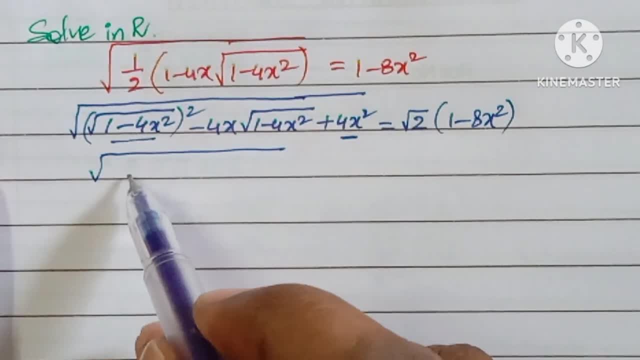 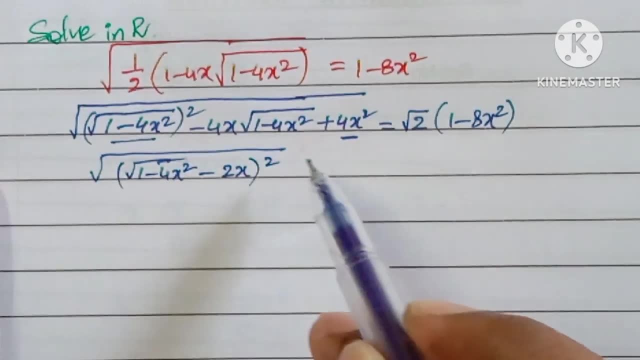 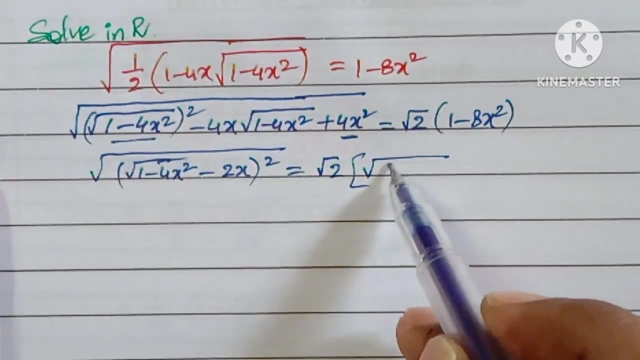 so here you will get a root of root of 1 minus 4 x square minus 2x whole squared a minus b whole whole square. Now this can be written as root 2 into root of 1 minus 4 x square whole square. 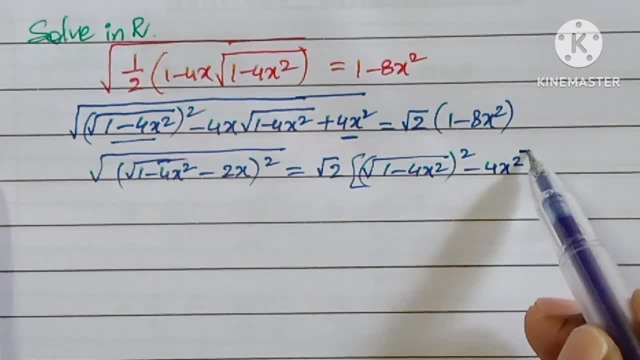 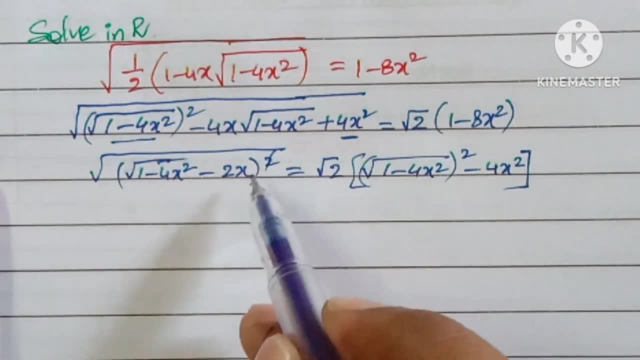 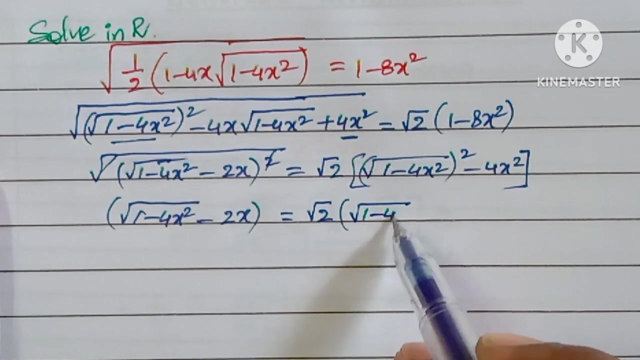 minus 4 x square. Now if you cancel this root root, you will get again 1 minus 8 x square. Now here square root and root get cancelled. Square root of 1 minus 4 x square minus 2 x is equal to root 2 into root of 1 minus 4 x square minus 2 x. into root of 1 minus 4 x square. 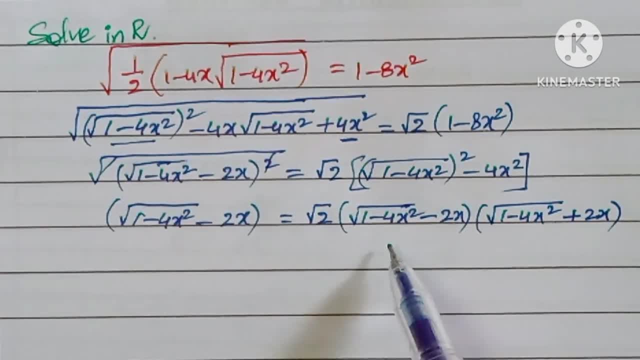 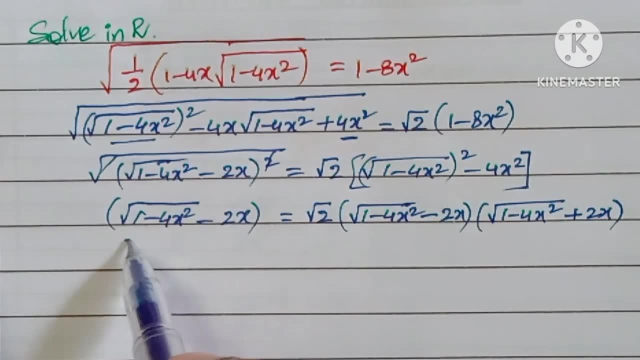 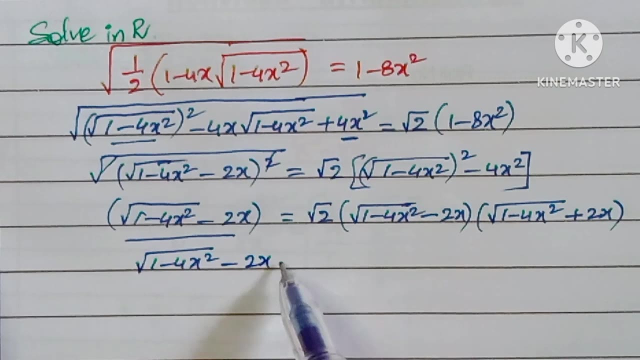 plus 2 x. Now here you are writing it as a minus b into a plus b. Now here you can take 1 minus this one as common. So here root of 1 minus 4 x, square minus 2 x is equal to 0. or you can write it as root 2 of. 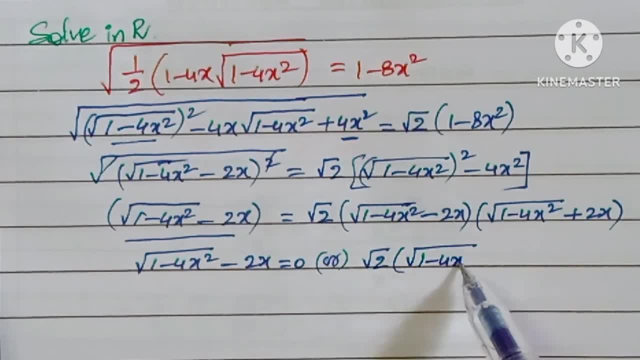 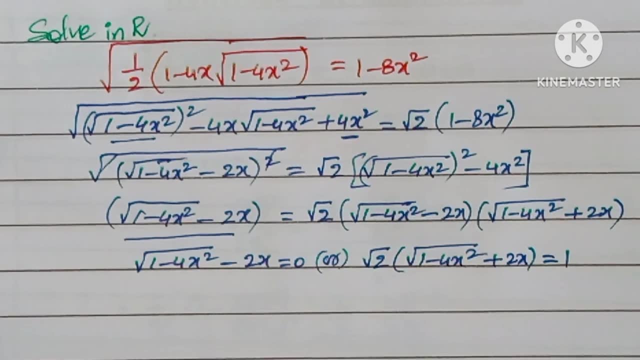 root of 1 minus 4 x square plus 2 x is equal to 1.. There you get two cases. Now you will go to the first case. root of 1 minus 4 x square is equal to 2 x, Now squaring on both sides. 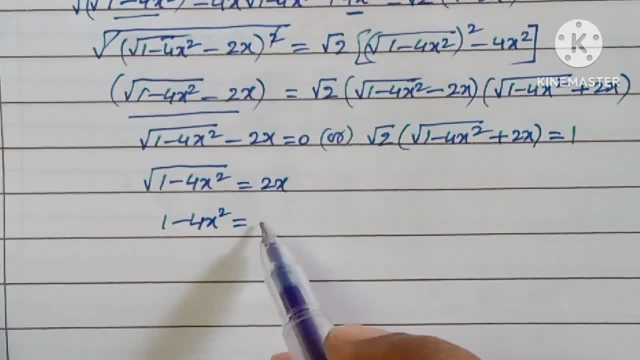 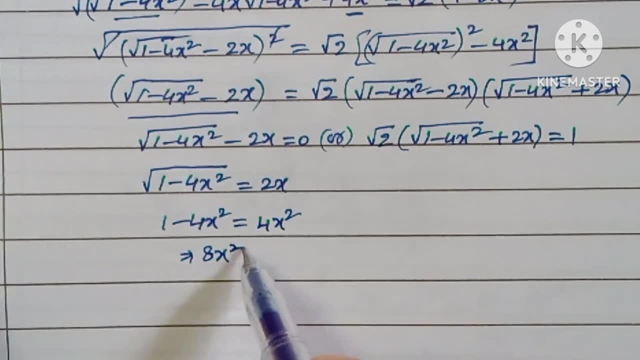 1 minus 4 x square is equal to 4 x square. That implies 8 x square is equal to 1 x square is equal to 1 by 8.. So this can be written as x square equal to 1 by 2 root 2.. Now, if you multiply with: 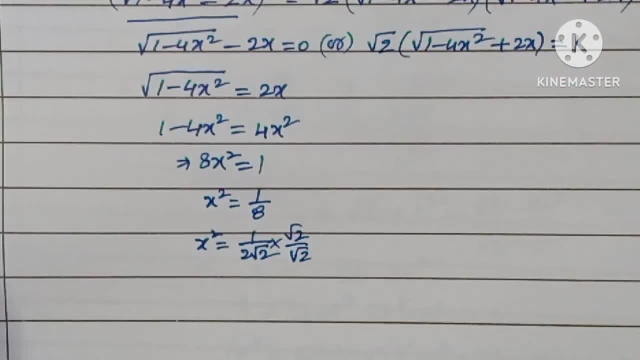 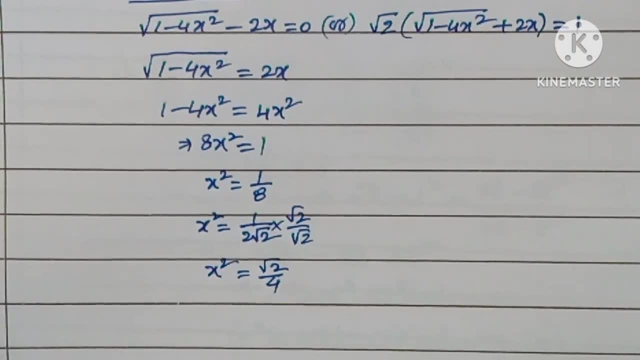 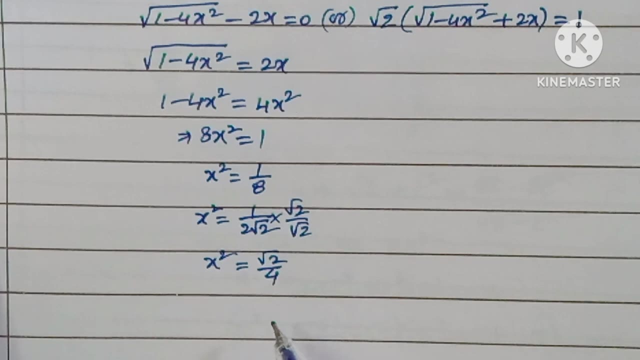 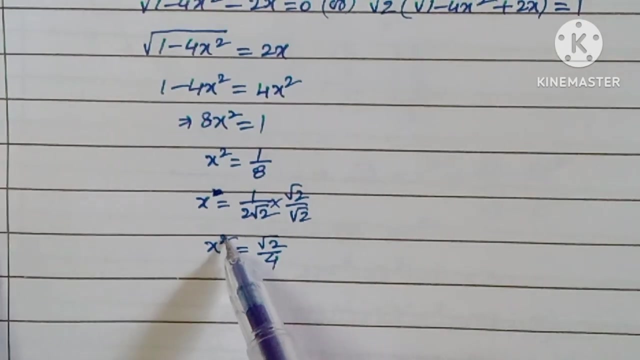 root 2 and rationalize it. x square is equal to root 2 by 4.. x square is equal to root 2 by 4.. Now here, x equal to 1 by 2 root 2.. So if you rationalize it, you will get root 2 by 4.. x value.